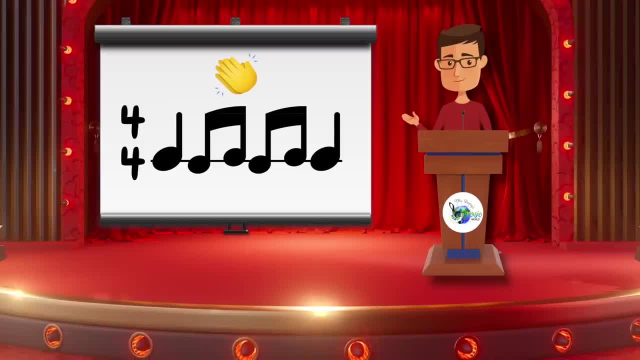 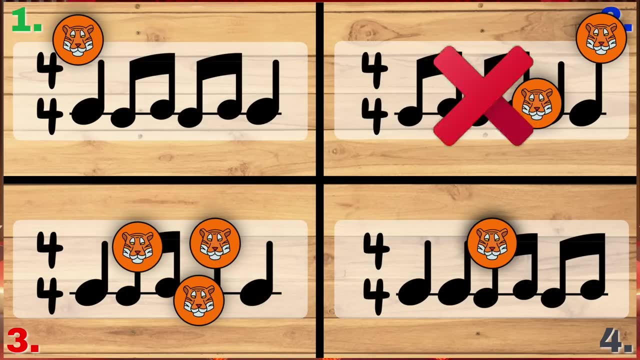 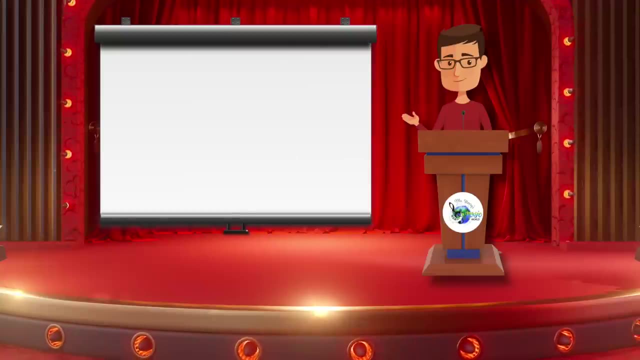 Once you are in the corner of your choice, a rhythm will be performed. If you are standing in the corner of the rhythm that was performed, then you are out of the game. Sorry, Oh, and teachers. check the description box for more info. 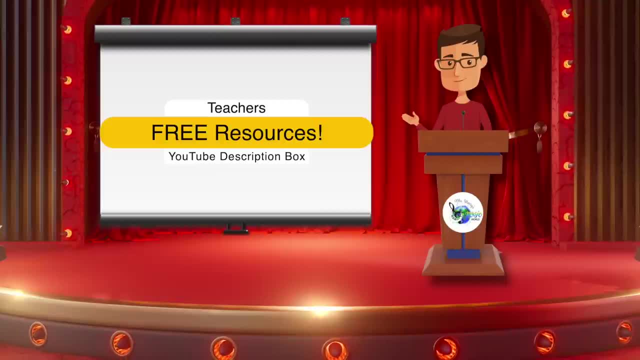 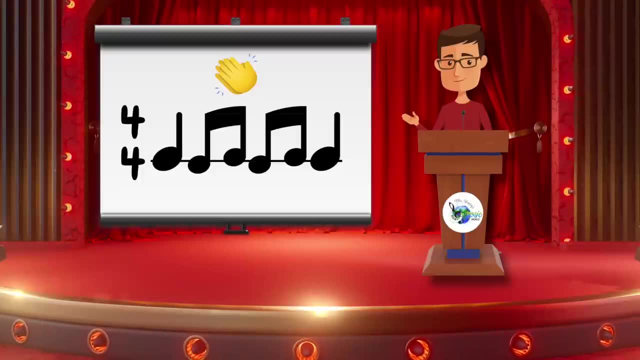 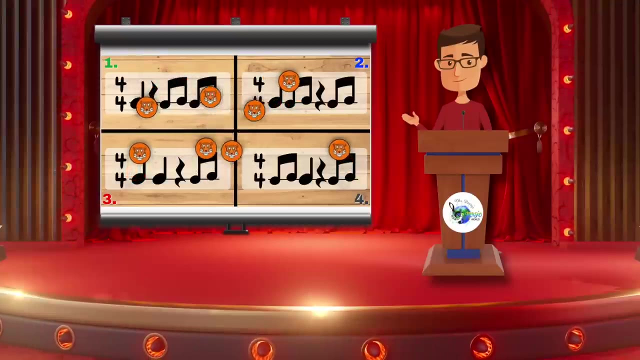 on how to get a couple free resources and extensions for this game for even more fun. Okay, back to the game. After the rhythm is revealed, the students who are out will simply take a seat and another 10 seconds will count down to allow you to pick a new corner. 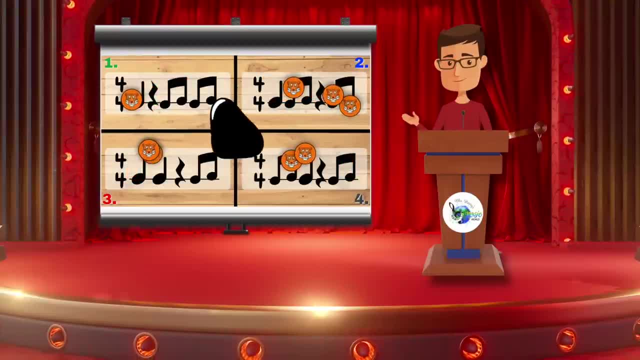 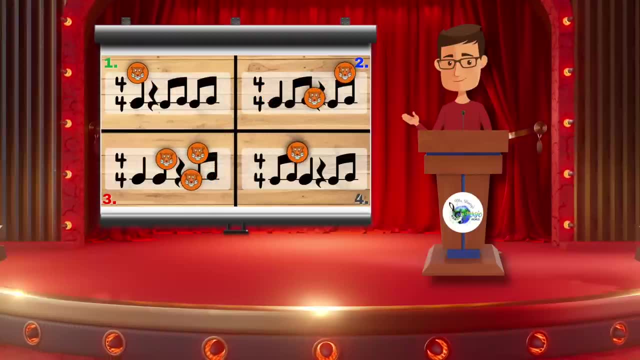 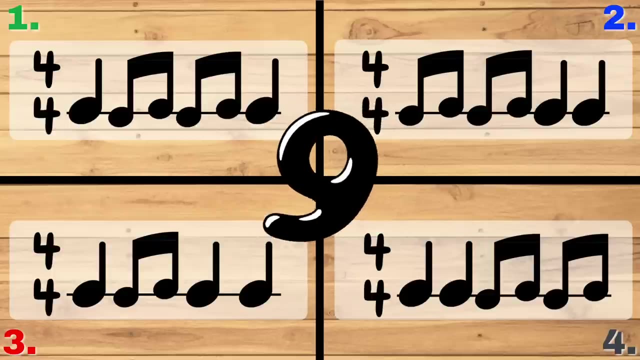 and the game will continue until there is one person left. So let's get started with the game. Ready set, go Find corner 1,, 2,, 3, or 4.. Aim for the ace. Okay, here is the rhythm. 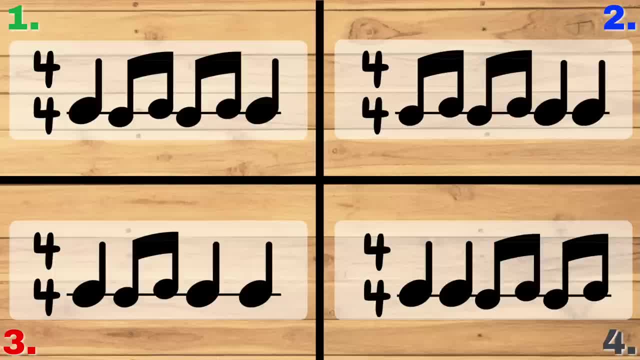 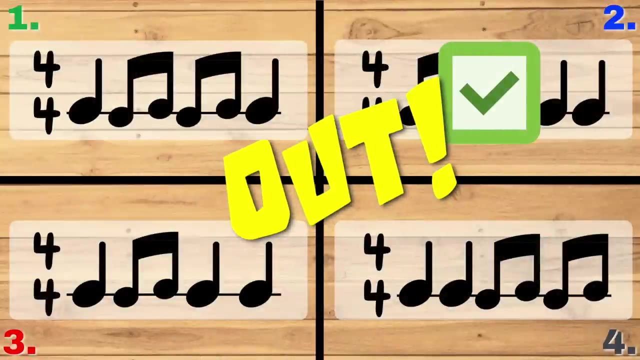 Let's listen again. Show with your fingers which corner the rhythm is in. If you said this corner, then you are correct. Take a seat because you are out. Let's start the clock for the next round. Ready set go. 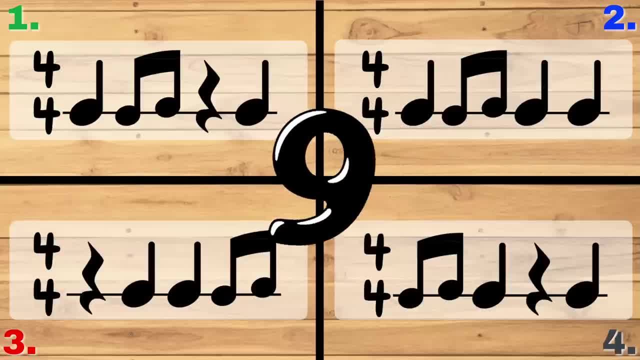 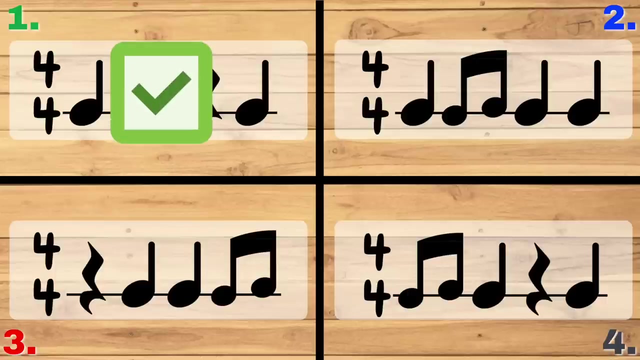 Ready set. go Find corner 1,, 2,, 3, or 4.. Aim for the ace. Okay, here is the rhythm. Let's listen again. Show with your fingers which corner the rhythm is in. If you said this corner, then you are correct. Take a seat, because you are out. 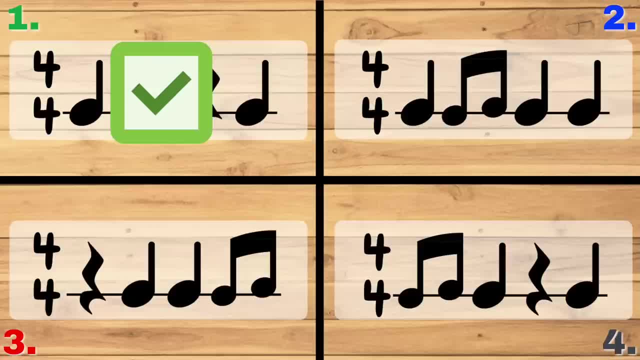 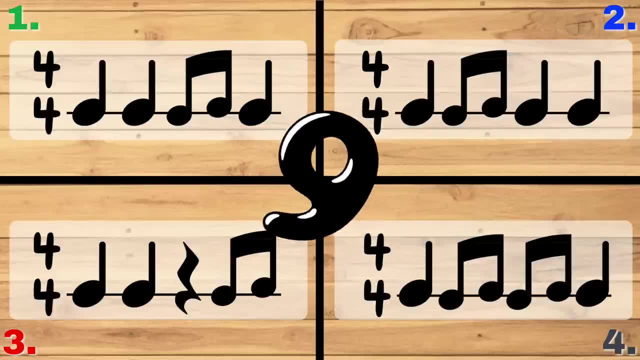 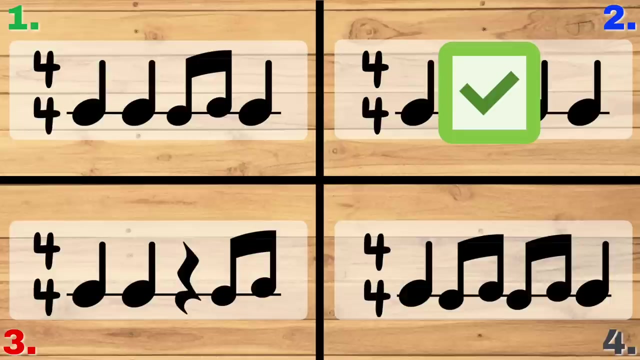 Let's start the clock for the next round. Ready set, go Find corner one, two, three or four. Okay, here is the rhythm. Let's listen again. Show with your fingers which corner the rhythm is in. If you said this corner, then you are correct. Take a seat, because you are out. 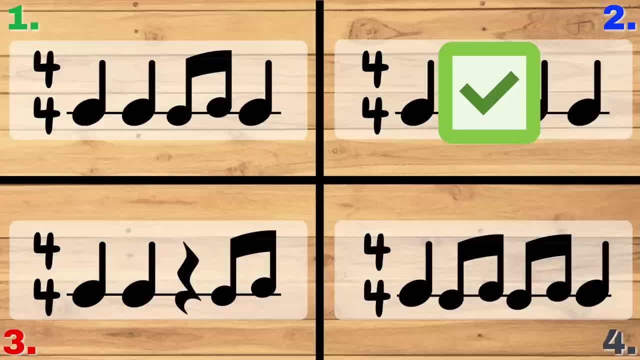 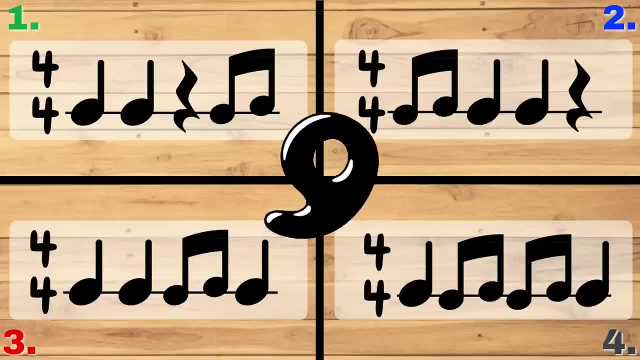 Let's start the clock for the next round. Ready set, go Find corner one, two, three or four. Aim for nice. Okay, here is the rhythm. Let's listen again. Show with your fingers which corner the rhythm is in. 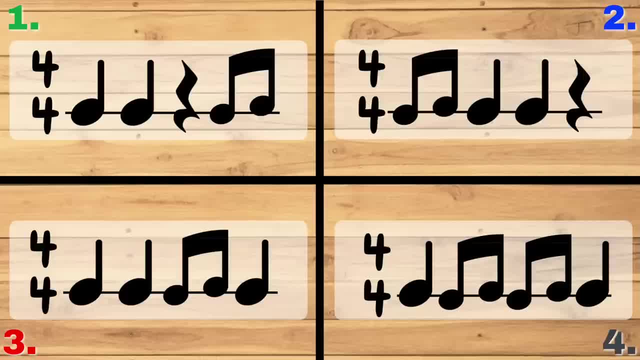 If you said this corner, then you are correct. Take a seat because you are out. Oh no, Let's start the clock for the next round. Ready, set, go? Find corner one, two, three or four. Aim for nice. 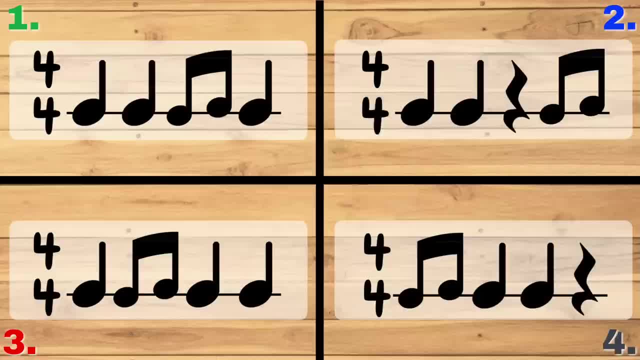 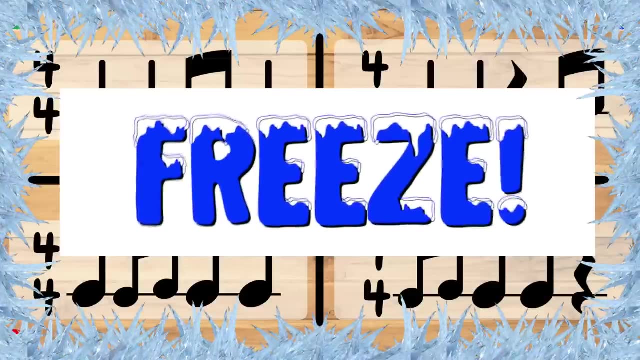 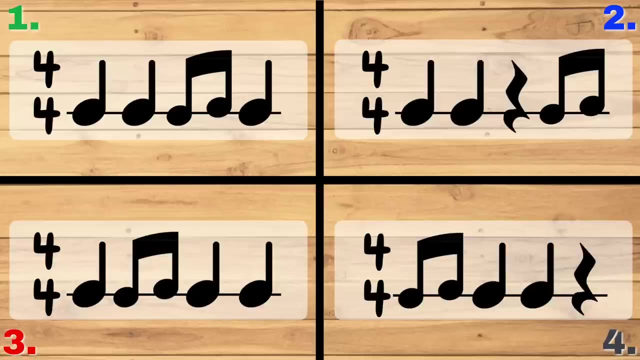 Show with your fingers which corner the rhythm is in. Okay, here is the rhythm. Let's listen again. Let's listen again. Oh no. And the last round. Show with your finger which corner the rhythm is in. Okay, here is the rhythm. 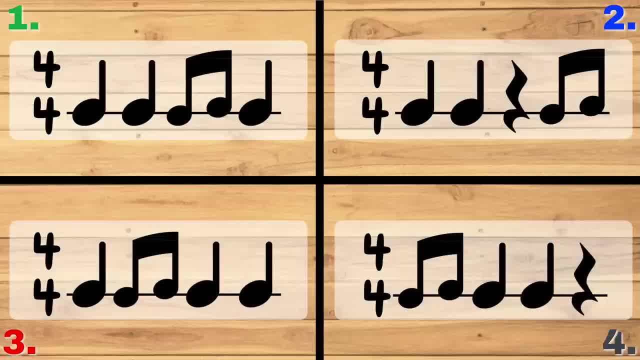 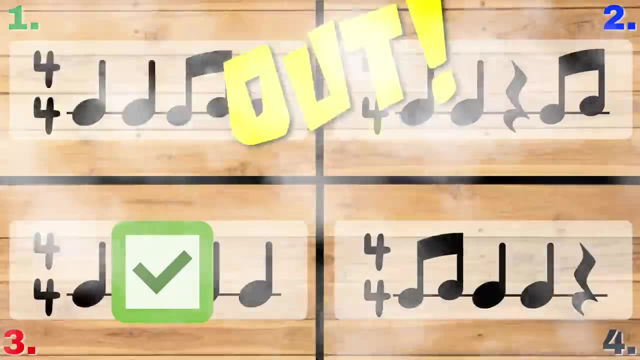 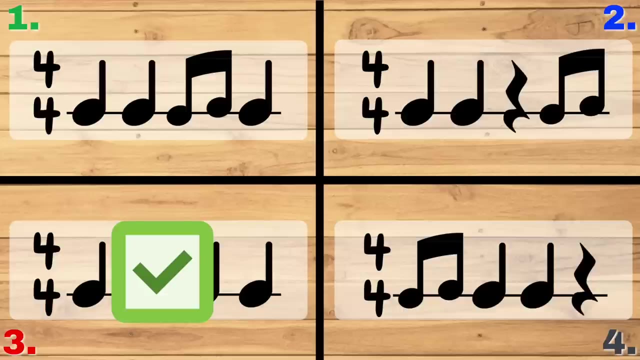 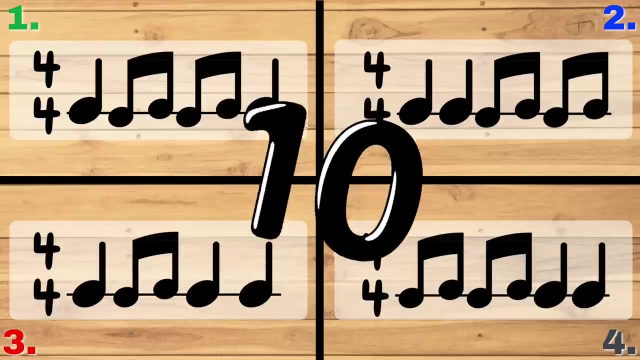 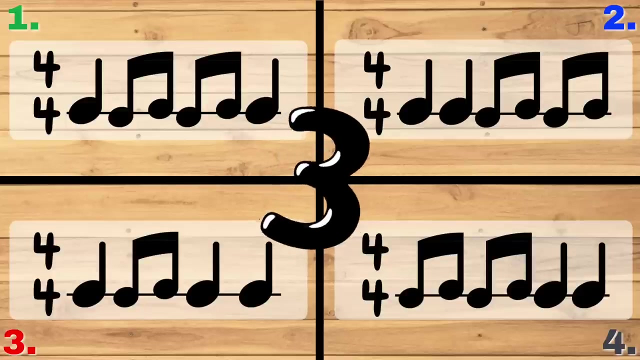 Show with your fingers which corner the rhythm is in. If you said this corner, then you are correct. Take a seat because you are out. Let's start the clock for the next round. Find corner 1,, 2,, 3 or 4.. 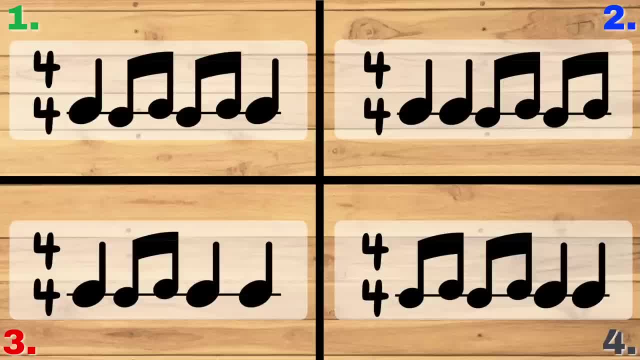 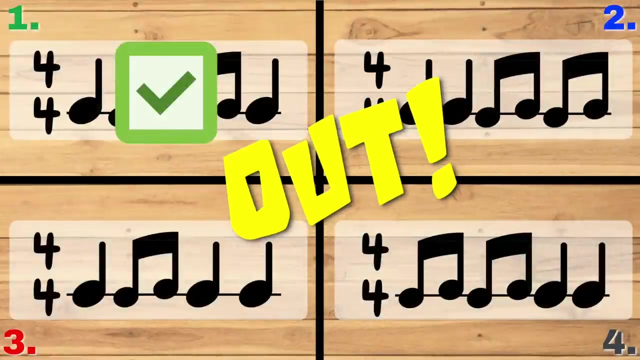 Okay, here is the rhythm. Let's listen again. Show with your fingers which corner the rhythm is in. If you said this corner, then you are correct. Take a seat, because you are out. Let's start the clock for the next round. 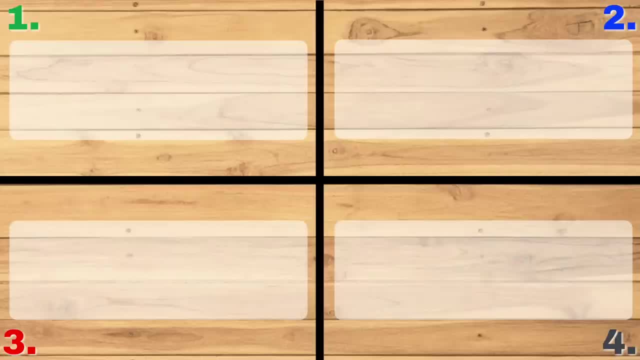 Find corner 1,, 2, 3 or 4.. Okay, here is the rhythm. Let's listen again. Show with your fingers which corner the rhythm is in. If you said this corner, then you are out. Let's start the clock for the next round. 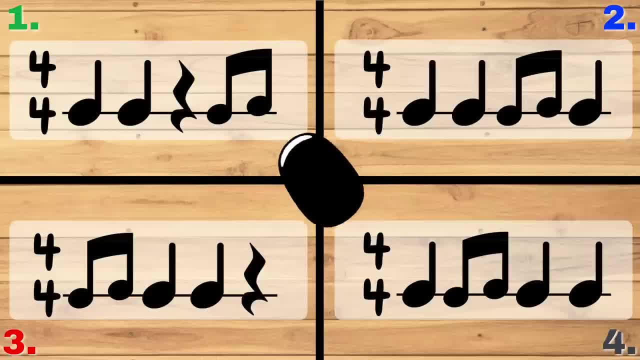 Find corner 1,, 2, 3 or 4.. Okay, here is the rhythm. Let's listen again. Show with your fingers which corner the rhythm is in. If you said this corner, then you are out. Let's start the clock for the next round. 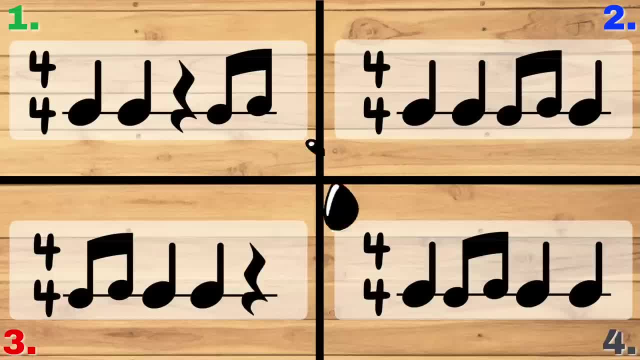 Find corner 1,, 2,, 3 or 4.. Okay, here is the rhythm. Let's listen again. Show with your fingers which corner the rhythm is in. If you said this corner, then you are out. Let's listen again. 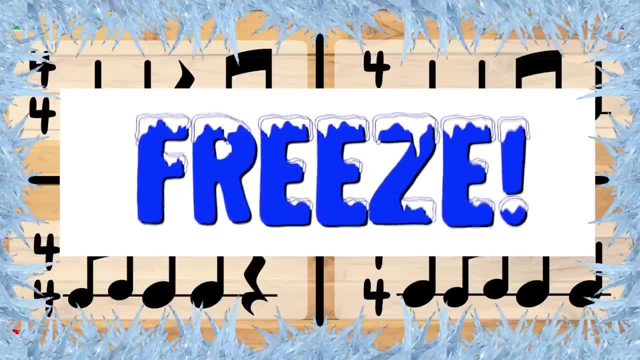 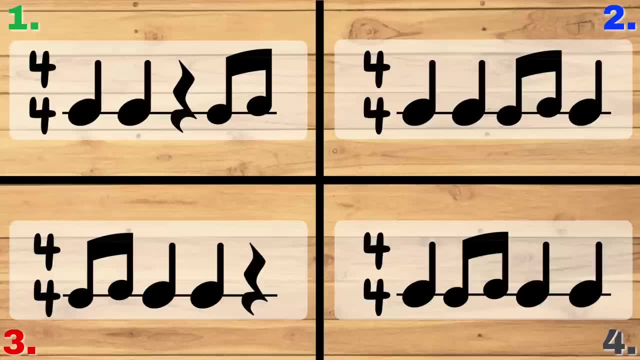 Show with your fingers, which corner the rhythm is in. If you said this corner, then you are out. Let's start the clock for the next round. Wow, that was a whole lot of speed again. Let's listen again. Show with your fingers, which corner the rhythm is in. 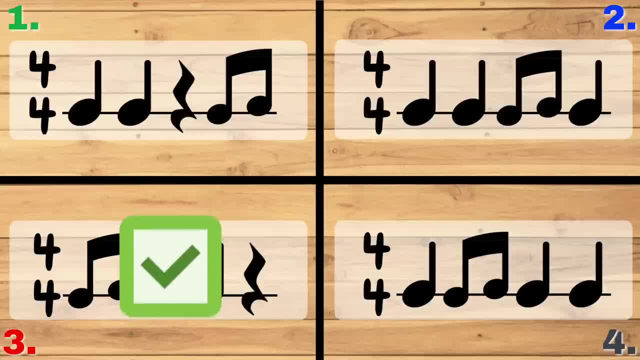 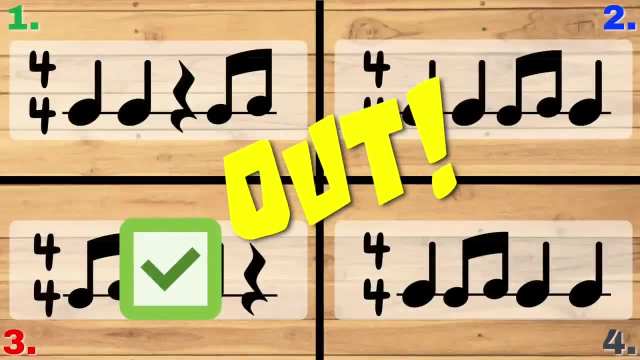 If you said this corner, then you are correct. Find corner, 3. Find corner. 4. Find corner. 5. Find corner. 6. Find corner. 7. Find corner. 8. Find corner. 9. What is this? Ready set go. 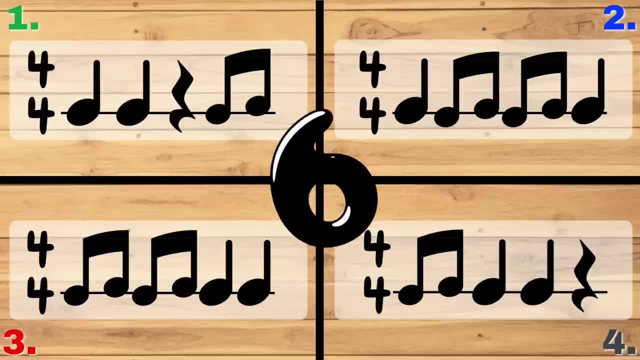 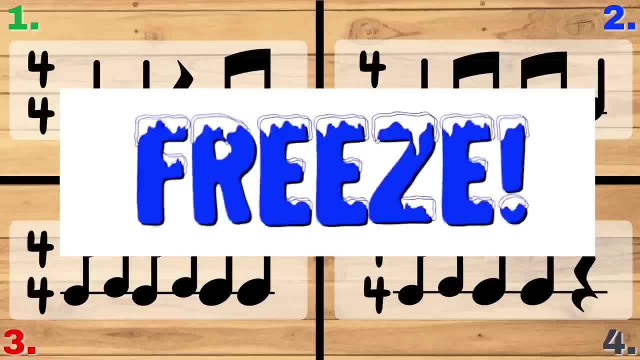 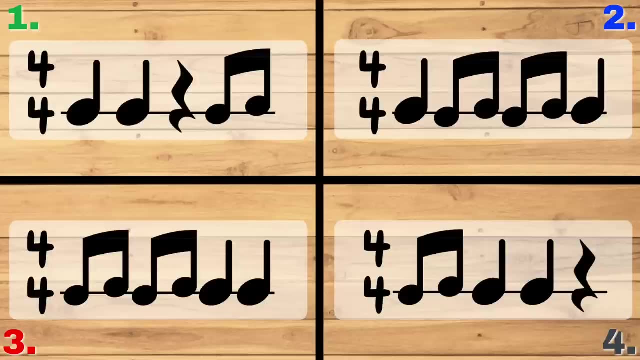 Find corner 1,, 2,, 3, or 4.. Aim for the ice. Okay, here is the rhythm. Let's listen again. Show with your fingers which corner the rhythm is in. If you said this corner, then you are correct. 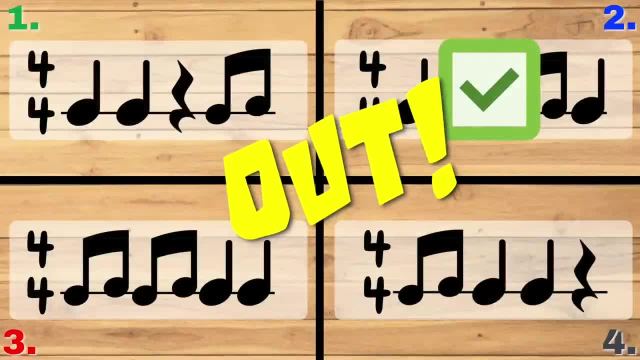 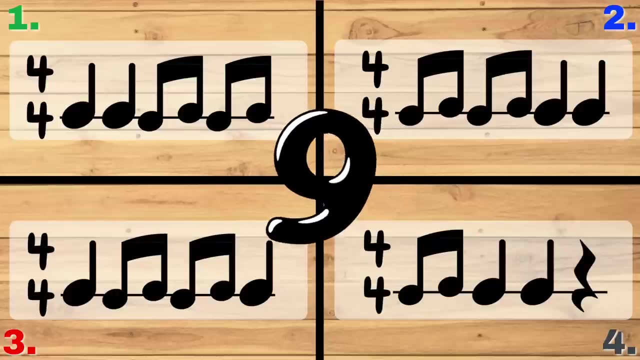 Take a seat because you are out. Let's start the clock for the next round. Ready set go. Ready set go Set go. Find corner 1,, 2,, 3, or 4.. Aim for the ice. 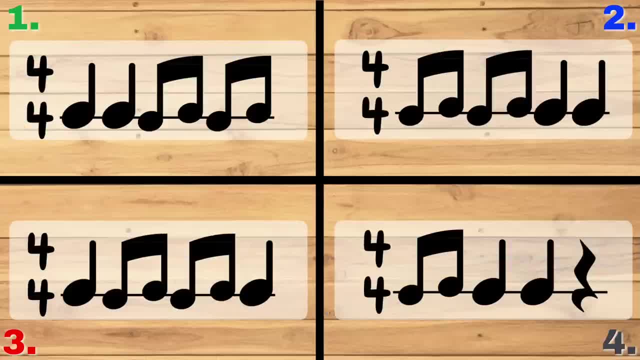 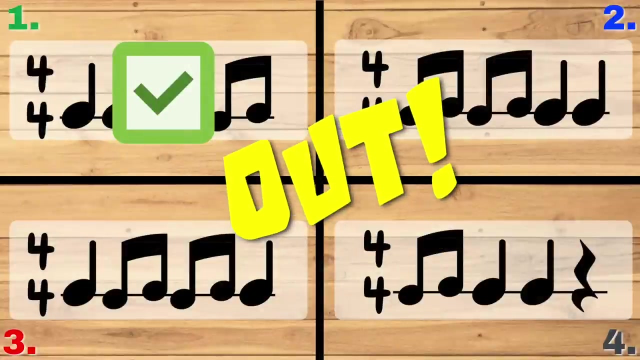 Okay, here is the rhythm. Let's listen again. Show with your fingers which corner the rhythm is in. If you said this corner, then you are correct. Take a seat because you are out. Oh no, Let's start the clock for the next round. 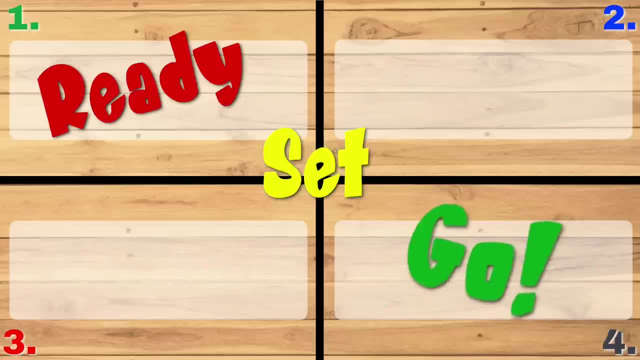 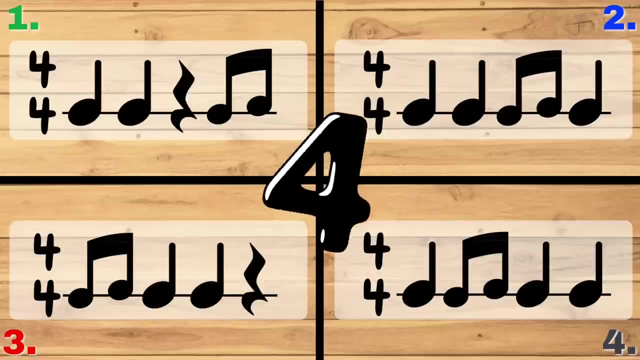 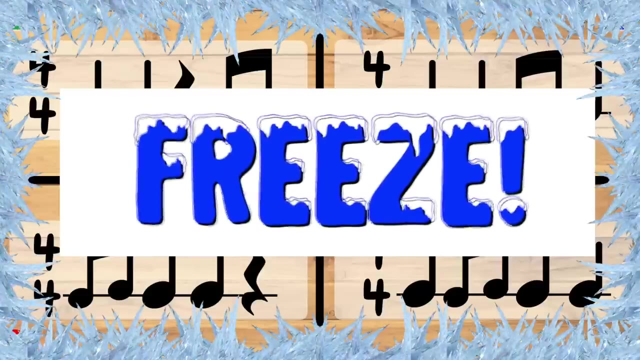 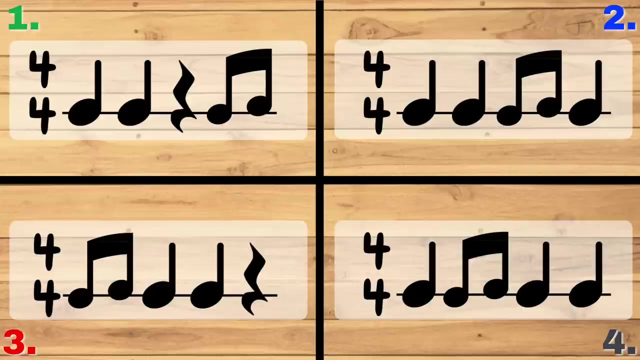 Ready set. go. Find corner 1,, 2,, 3, or 4.. Aim for the ice. Okay, here is the rhythm. Let's listen again. Show with your fingers which corner the rhythm is in, fingers which corner the rhythm is in. 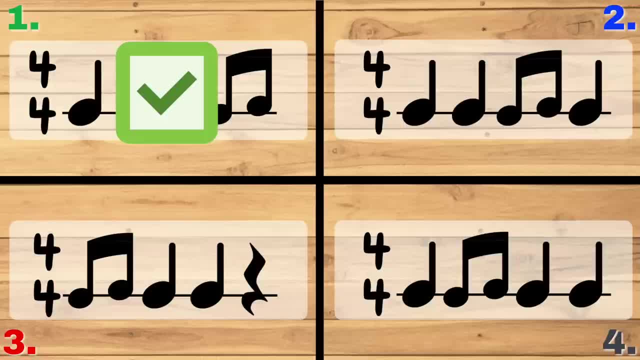 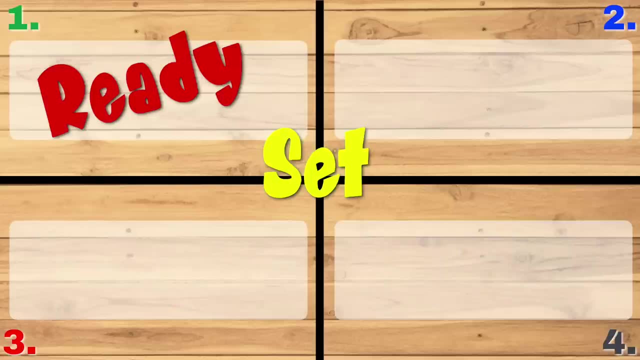 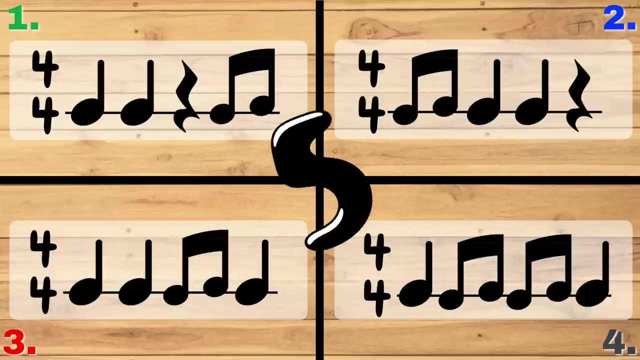 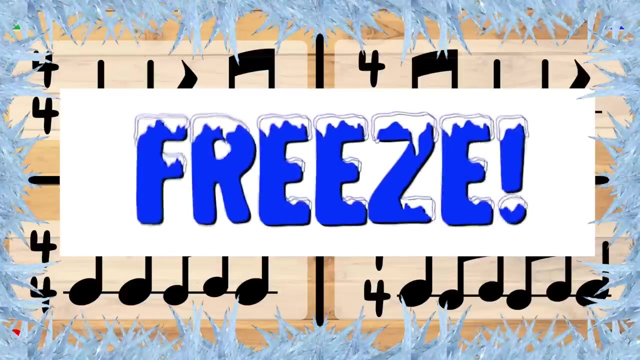 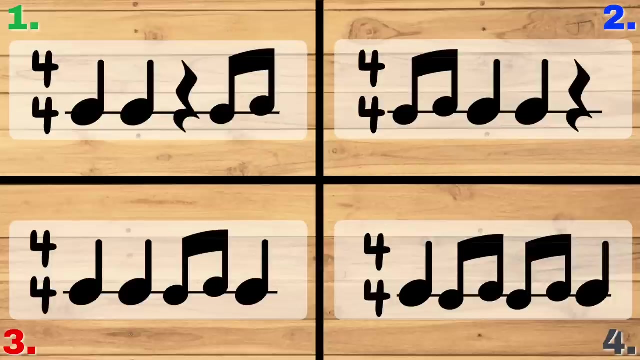 If you said this corner, then you are correct. Take a seat because you are out. Let's start the clock for the next round. Find corner 1,, 2, 3 or 4.. Okay, here is the rhythm. Let's listen again. 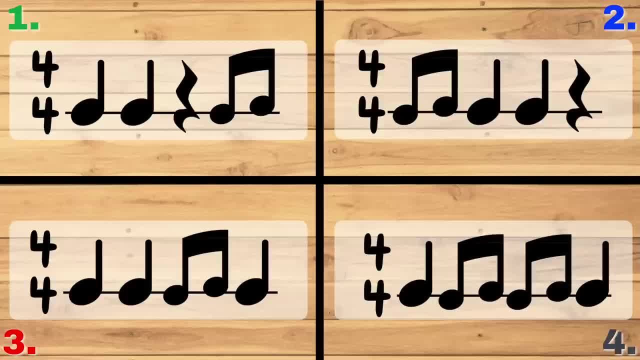 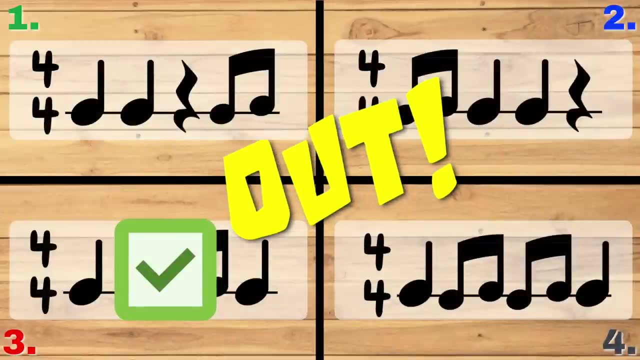 Show with your fingers which corner the rhythm is in. The rhythm is in. If you said this corner, then you are correct. Take a seat because you are out. Let's start the clock for the next round. Find corner 1,, 2,, 3 or 4.. 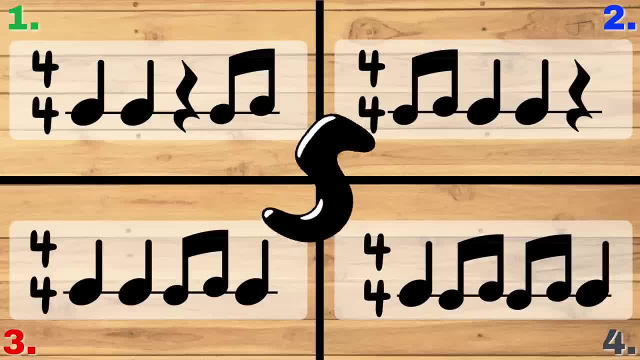 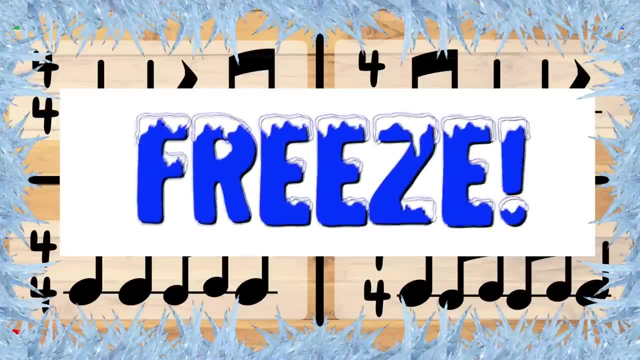 Okay, here is the rhythm. The rhythm is in. Okay, here is 4. The rhythm is 4. The rhythm is 5. 1, 2, 3, 4- Let's start the clock- 3 or 4.. Okay, here is the rhythm. 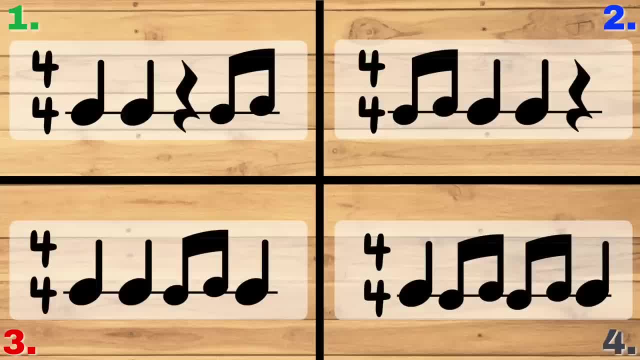 Let's listen again One more time. The rhythm is in. The rhythm is in One more time: 3 or 4.. The rhythm is in 3 or 4.. If you said this corner, then you are correct. 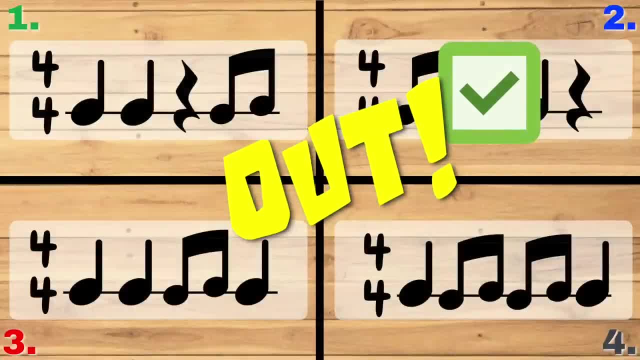 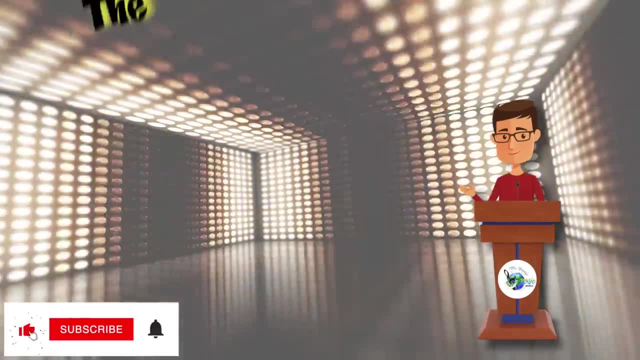 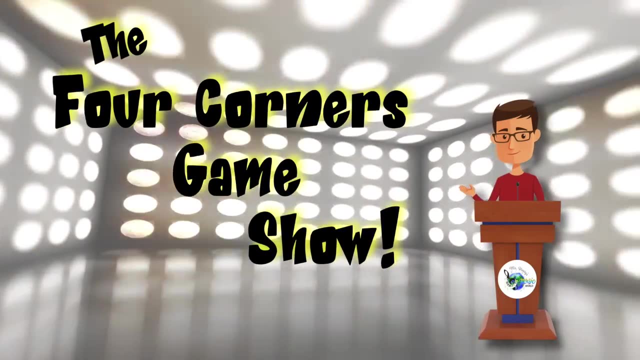 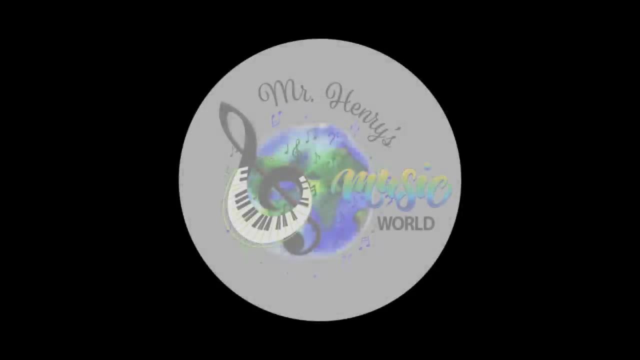 Take a seat because you are out. Oh no, The Four Corners Game Show. The Four Corners Game Show.